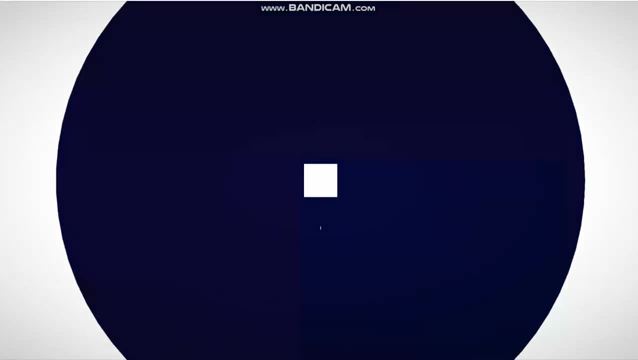 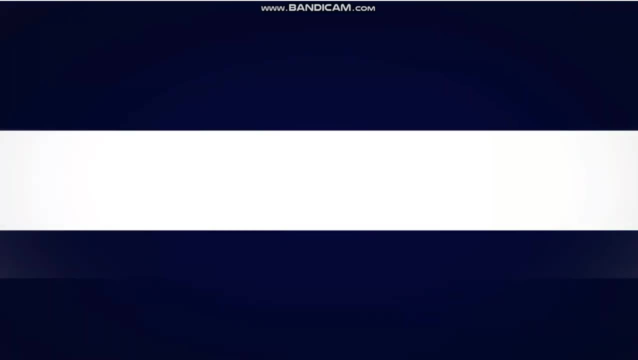 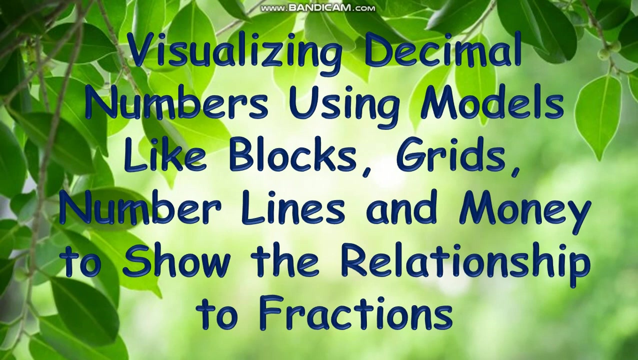 Hello, how are you? Are you ready for our lesson again today? If your answer is yes, be prepared, focus and learn more. What we are discussing today is visualizing decimal numbers using models like blocks, grids, number lines and money to show the relationship to 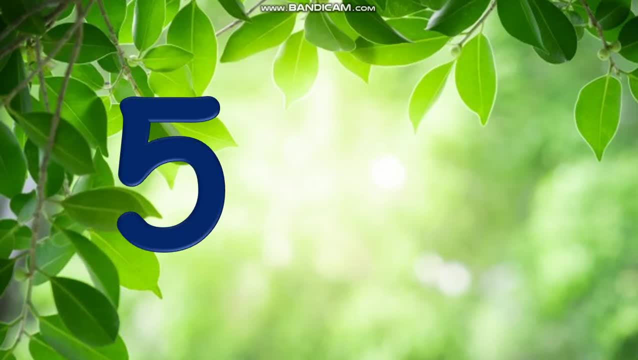 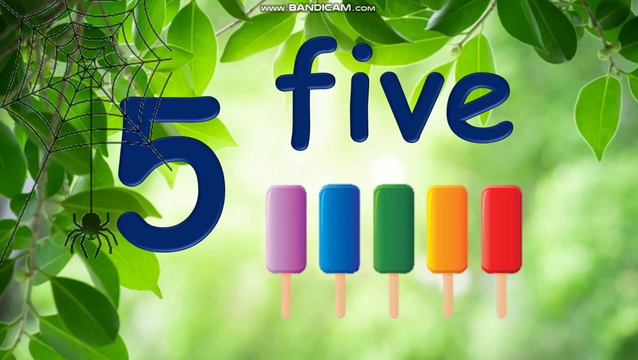 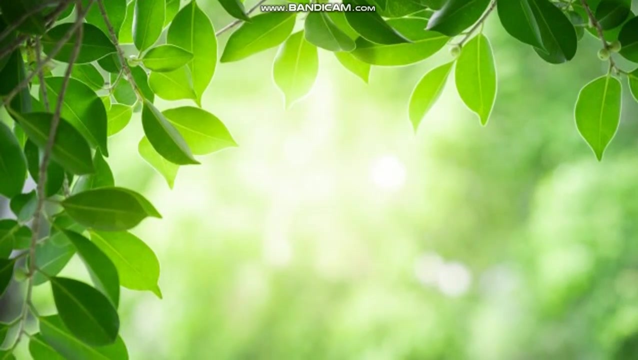 fractions. What number do you see? If you see 5, you know that it means 5 objects or 5 units, right? How about this number? Do we read it simply as 0.5?? Is there any other way to read it correctly? 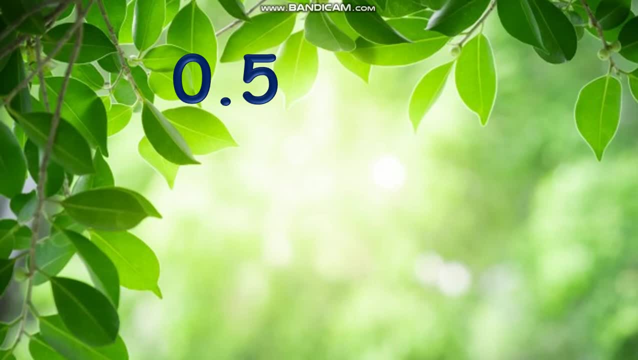 The number 0.5 or 0.5 is a decimal and is just a number. A decimal is just another way of writing the fraction 5 tenths, As a rule. a decimal is just another way of writing fractions whose denominators are powers of 10, and the proper way to read them. 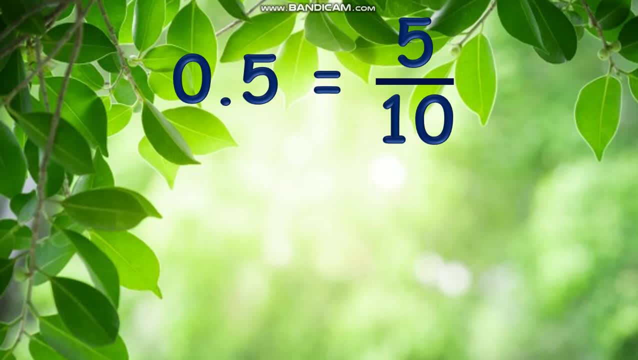 is the same as reading the equivalent fractions they represent. Let us visualize 0.5 with the place value chart of our number system, which now includes the decimals, And since 5 tenths is our fraction, we can read it as 0.5.. If you see 5, you know that it means 5 objects or 5 units. 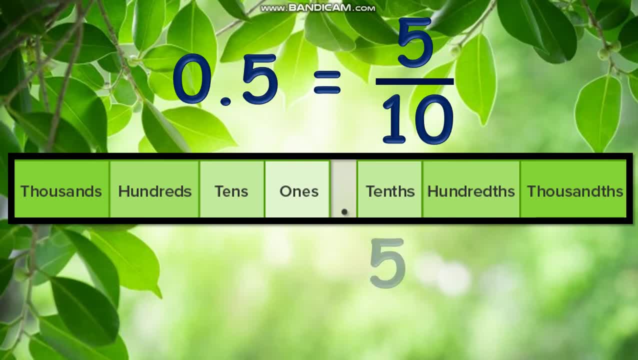 and that is why it is written as a decimal. This is how you use the decimal function. So let us visualize this decimal function. The decimal function is in the column of tenths place with the decimal point on its left, and next is the whole number 0.. Therefore, we can now read this: 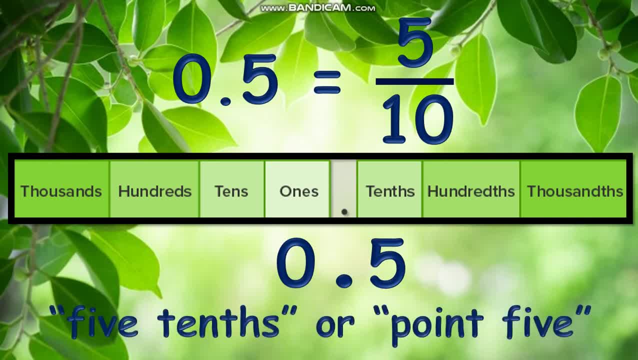 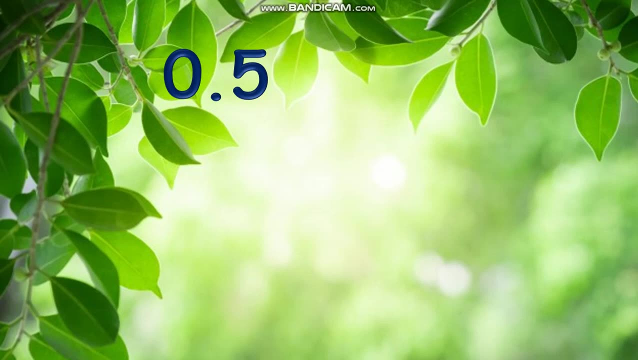 decimal as 5, tenths or 0.5.. One way to visualize a decimal is to use blocks or grids. An example is the decimal function. If you see a decimal in the column of tenths, place with the decimal diagram. Since 0.5 in a fraction is 5 tenths, we simply visualize it by a. 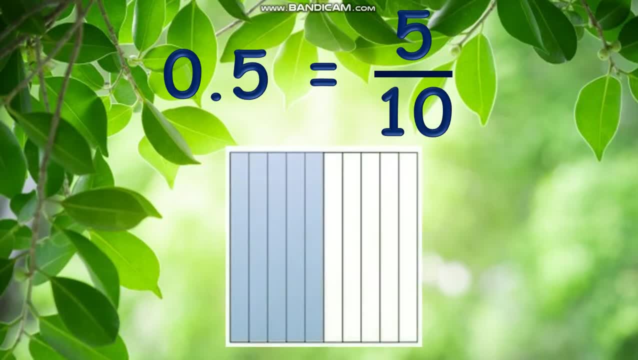 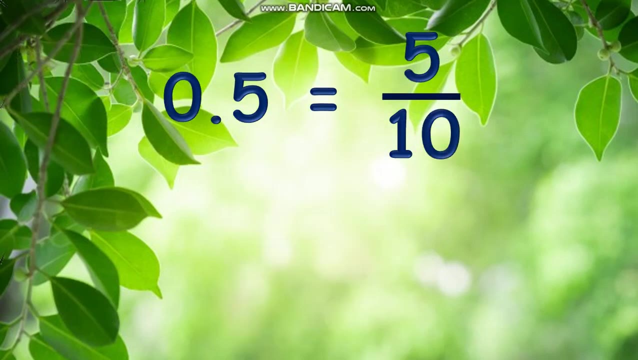 fraction of 5 tenths. 5 shaded parts out of 10 equal parts To represent 0.5 or 5 tenths on a number line. divide the segment between 0 and 10 into 10 equal parts. The arrow jumps 5 equal parts from 0 to where it points lands at 0.5 and. 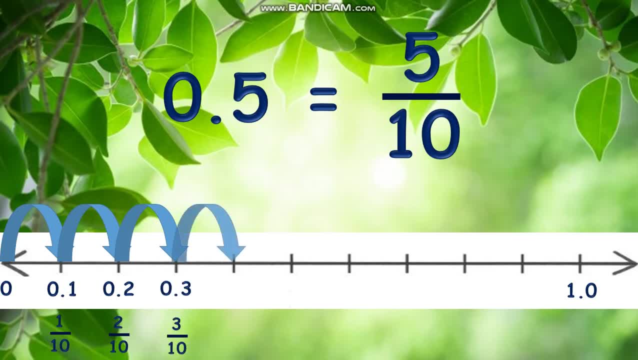 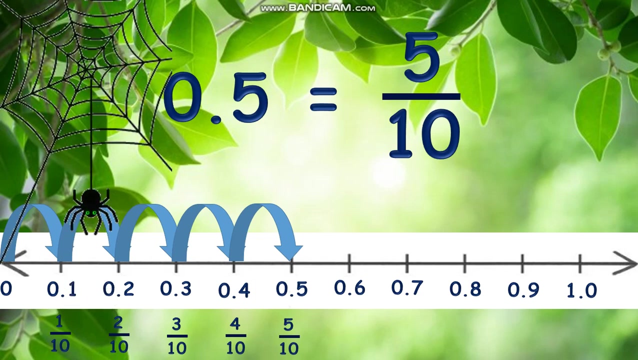 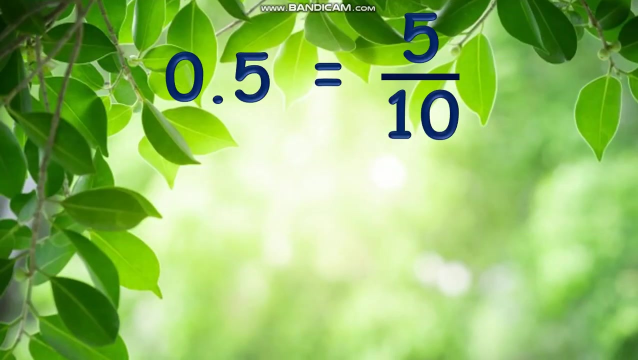 equal to 5 tenths, or 5 tenths For 1 half in fraction form. The relationship among pesos, bills, coins and centavos is a good model for decimal numeration. How can we visualize the decimal 0.5 with money? 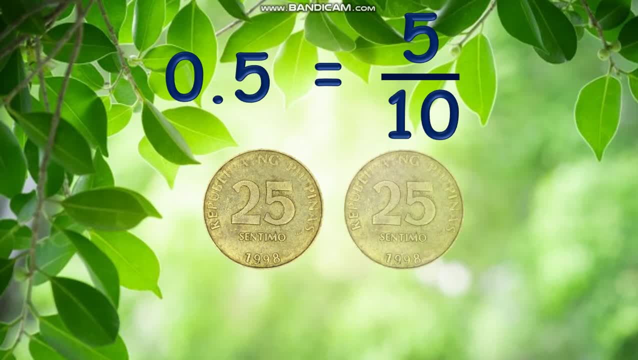 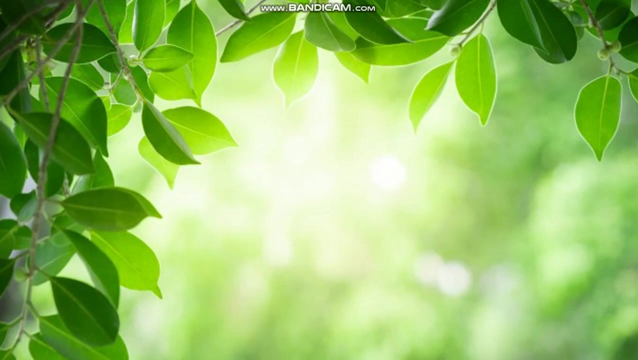 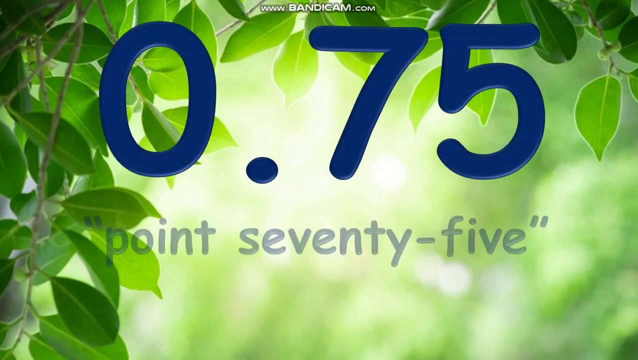 Simply 2: 25 centavos equals to 50 centavos, or 0 pesos and 50 centavos- The head of the decimal- is a piece of rock. Let's have another example of decimal: 0.75 or 75 hundredths. 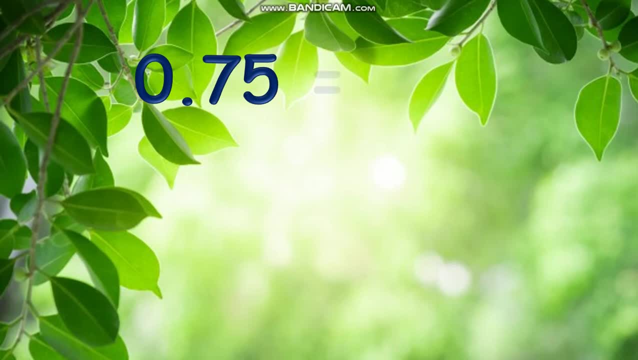 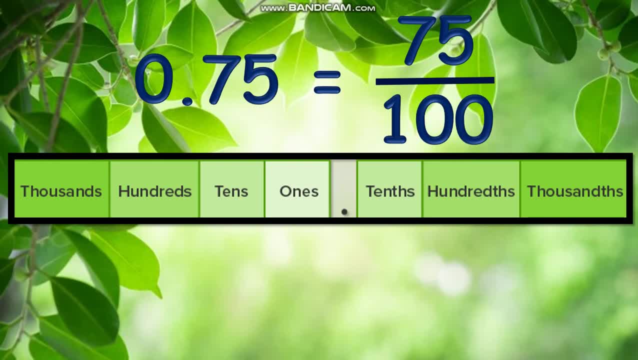 And since seventy-five hundredths is our fraction, seven is in the column of tenths place. Five is in the hundredths place with the decimal point on the left of seven. next is the whole number zero. Therefore, we can now read this decimal as seventy-five hundredths or point seventy-five.